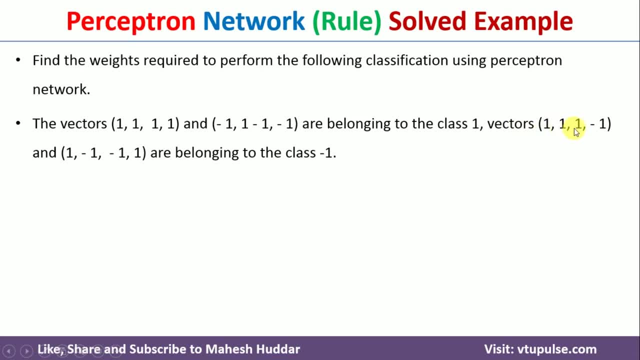 belongs to class 1, and the next vector is 1: 1, 1 minus 1 and 1 minus 1 minus 1: 1. These two belongs to class minus 1 in this case. Now, given this particular data points, we need to use the 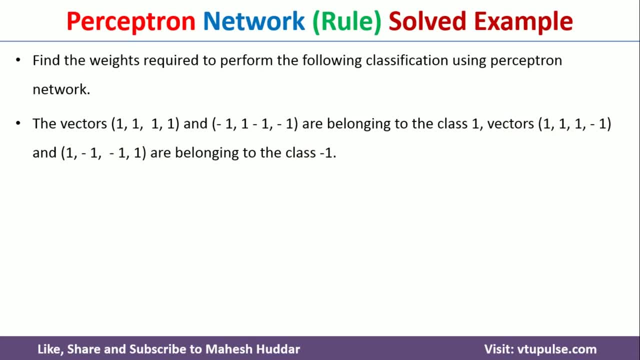 perceptron learning rule and find the optimal weights, They classify this particular data properly. So first we will assume the learning rate for this particular numerical example as 1 here, and we will initialize all the weights, including bias, to 0 in this case. So this is how the input data looks. 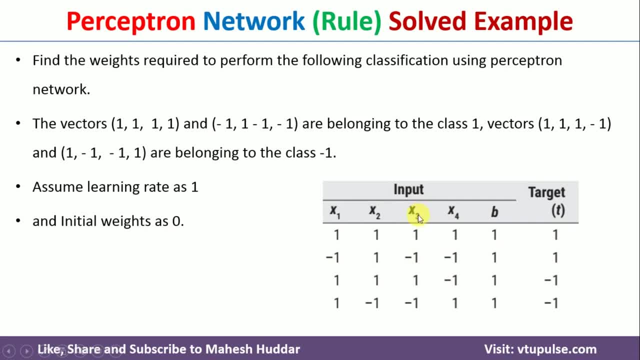 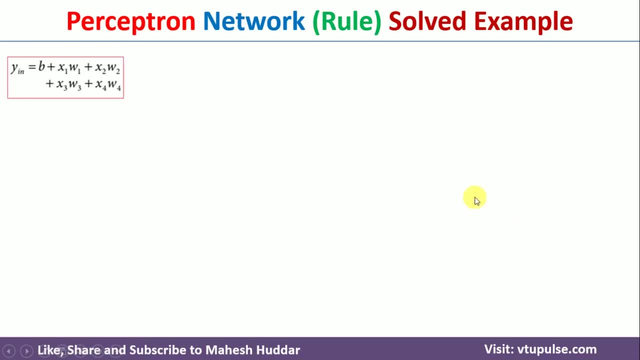 like Whatever has been given that has been written in the form of a table over here. Here we have four inputs and t is the target over here. Now, if you want to use the perceptron learning rule, the very first thing what we need to do is we need to calculate the net input. 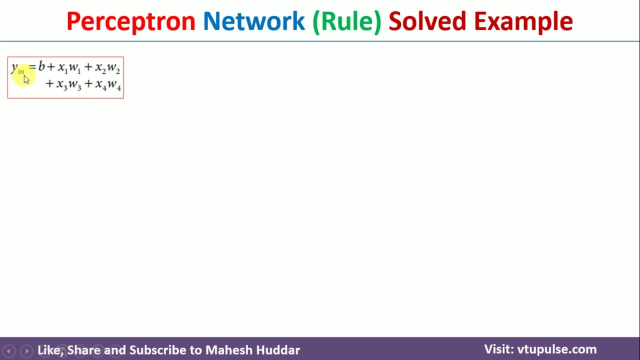 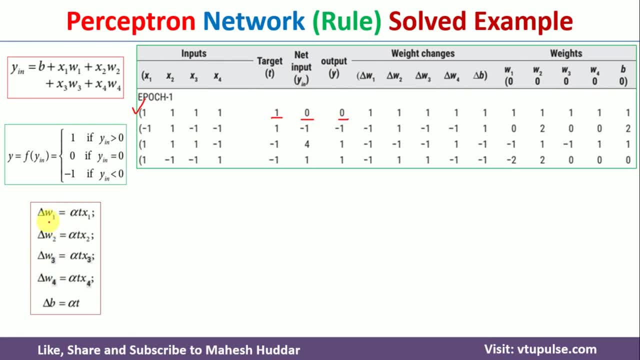 using the formula. So we need to calculate the net input to a particular neuron, that can be calculated the weights. So we need to calculate the change in weights first. the weight. So to calculate change in weights we have written: delta w1,, delta w2,, delta w3,, delta w4. 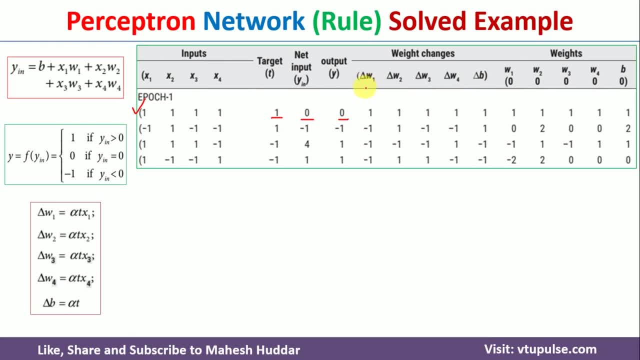 delta w5, delta w6, delta w6, delta w7yeah delta. we know the equation: nothing extension outside of delta w1. equation is alpha p x1. equation is alpha p x1. learning rate: learning rate. guess this table. guess this table one. 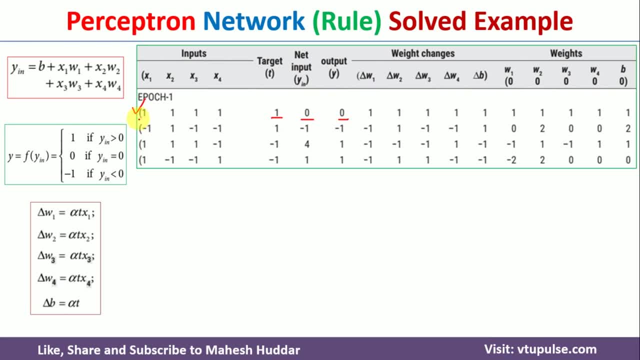 one. one thing will become 1 here. Similarly, I have to calculate delta w2.. Delta w2 is what Alpha, t, x2.. Alpha is known to us, that is 1. Target in this case is 1.. x2 is what Here x2 is equivalent to. 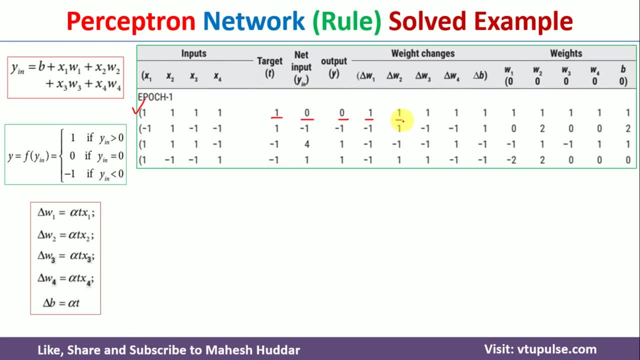 1 here. So once you calculate this one, you will get delta. w2 is also equivalent to 1 here. Similarly, we need to calculate delta w3, delta w4 and delta b. Once you calculate all these things, we need to calculate the change in weights. How to calculate the change in weights? w1- old is. 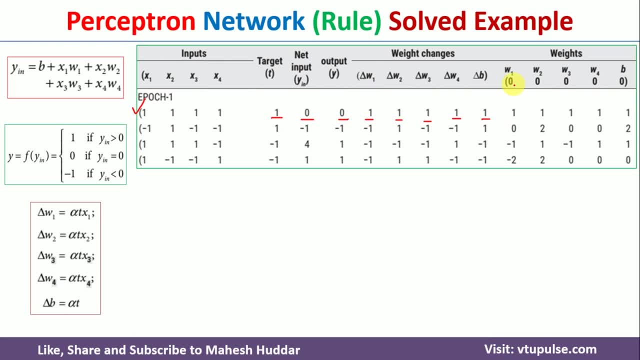 equivalent to 0.. w1 new is equivalent to w1 old plus delta w1.. So this is 0 plus 1, which is equivalent to 1 here. w2 new is equivalent to w2 old, that is 0.. Delta w2, that is 1.. So 0 plus. 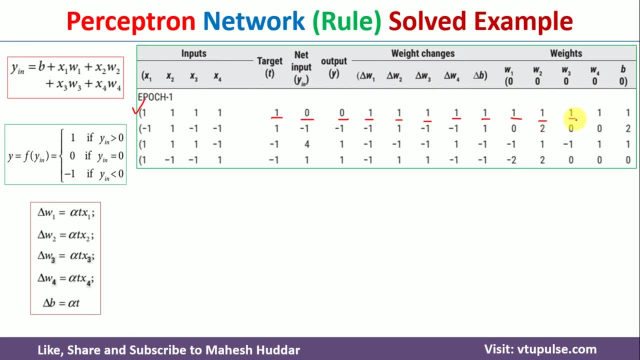 1 is equivalent to 1 in this case. Similarly, we need to calculate delta: w3 new, w4 new and then b- new in this case. Once you see this, do the calculation, you can see here. previously the weights were. 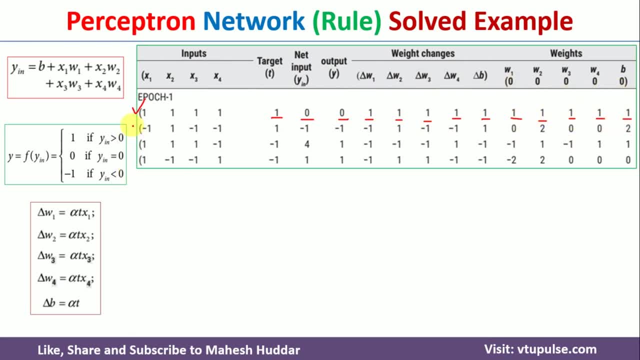 0. Now they were modified here. Now what I do is I will give the next input first. So this is the next input. Again, the target is known to us, that is 1, and we need to calculate the net. 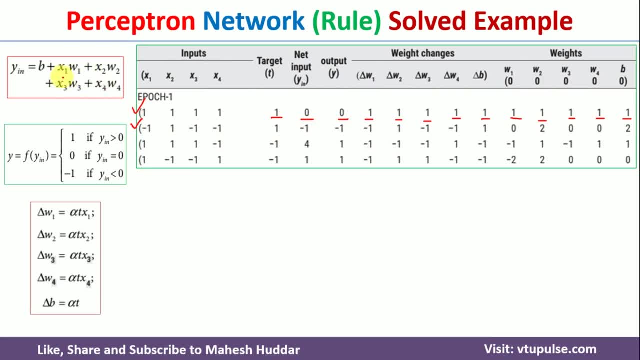 input here. So net input in this case is we need to use this particular equation to get the net input. If I put all the values, I will get minus 1 here, and if I use that activation function- that is, minus 1 is less than 0, I will get output as 1 in this case. So that is nothing but output. 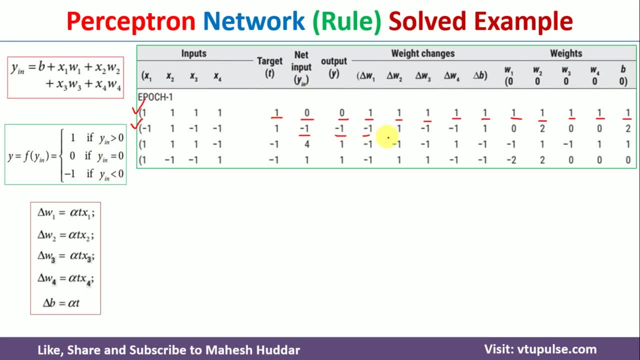 is not equivalent to target. here Again we have to calculate the weight updations here. So I will calculate all these things. I will add these things to the previous weights. that is, 1 is the old weight and delta w1 is equivalent to minus 1.. If I add these two things I will get 0. 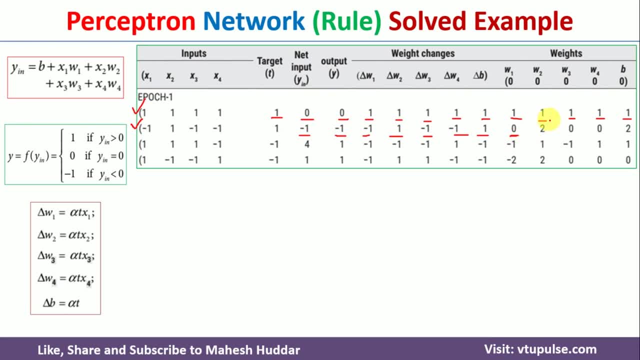 here Now: w2 new is equivalent to previous, one is 1, delta w2 is 1, 1 plus 1 is equivalent to 2.. Similarly, we have to calculate all these things. Next, we need to give this as the: 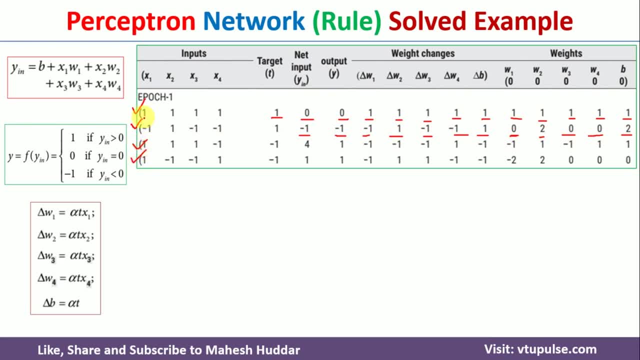 input and similarly we have to give this as the input to our neural network. So once all the four inputs were given, we have to see whether there was a change in weight in this particular iteration or not. Because there is a change in weights, we have to continue with one more. 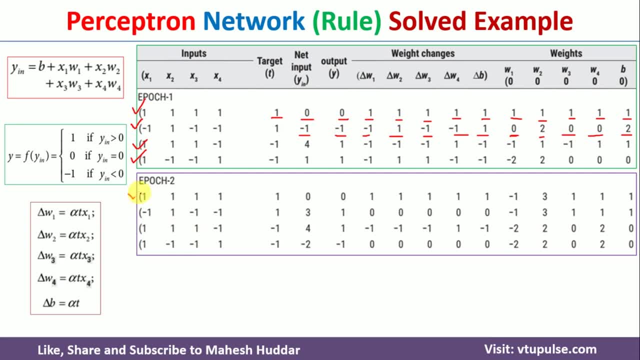 iteration. in this case, Again, we have to start with the first input. So we have to give this input to the system. We have to calculate the y in here, use this particular equation, and then we need to calculate the output. So, because it is equivalent to 0,, the output is equivalent to 0. 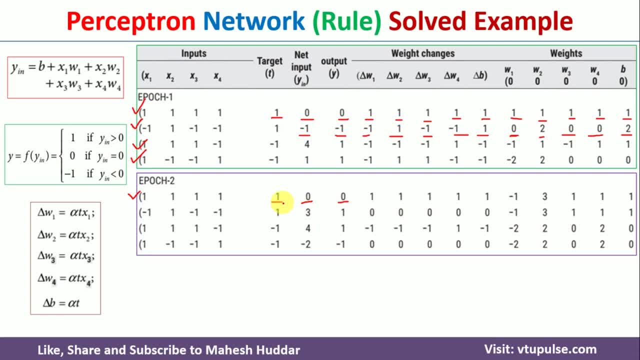 here. So this output is 0 and target is equivalent to 1. here They are not matching. Again, we have to calculate the delta terms. Once you calculate the delta terms, add these things to the previous weights. The last weight was minus 2, that is with respect to w1.. Minus 2 plus 1 will become 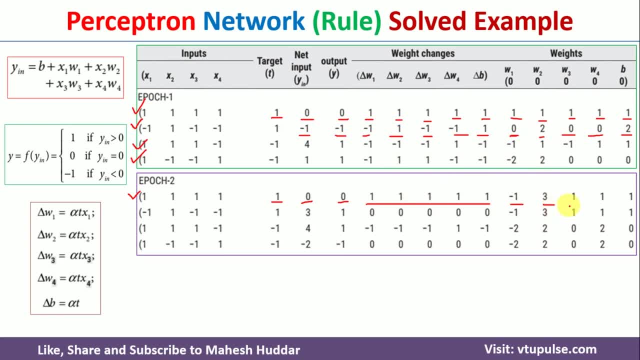 1 here, 2 plus 1, it will become 3 here. Similarly, we have to calculate all these things Again, we need to calculate y in and then y out. y is equivalent to target in this case. So there is. 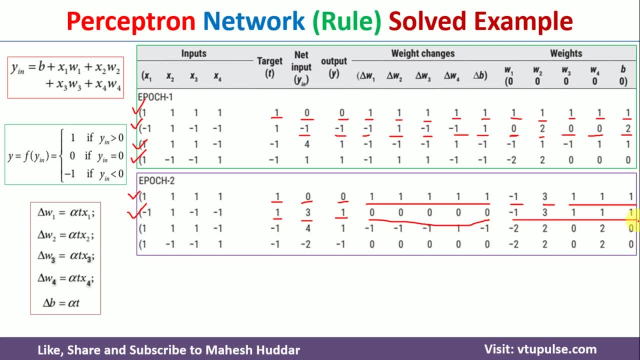 no need to do the weight updation. The previous weights will remain same here. I will give this as the input here and then I will calculate the y in. y in is equivalent to 4.. Because 4 is greater than 0,, output is 1.. Output is 1,, but target is minus 1.. They are not matching. Again we need to. 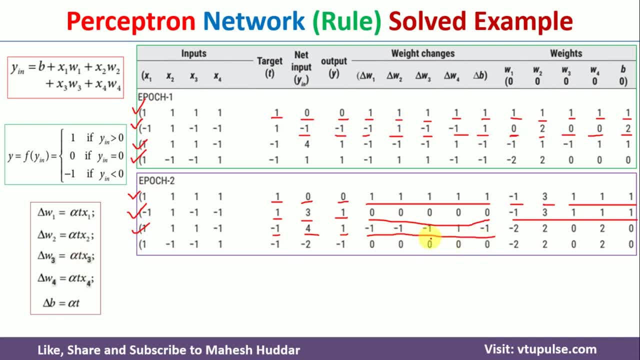 calculate the delta terms. The equation is given here: Using those things we calculate delta terms and then we will add these delta terms to the previous weights, So we will get the new weights here. I will give the fourth input. The y in is minus 2.. The output is minus 1 and the target is 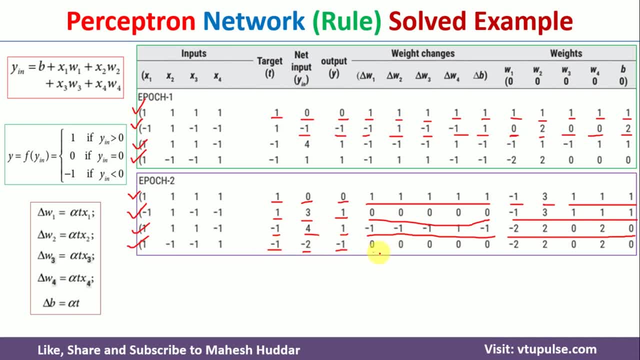 minus 1 here. Target and output is matching here, So no need to do the weight changes and the weights will remain same in this case. Again, if you look at this particular iteration or the second epoch, there was a change in weight. So what we do, We will try to go with another iteration or